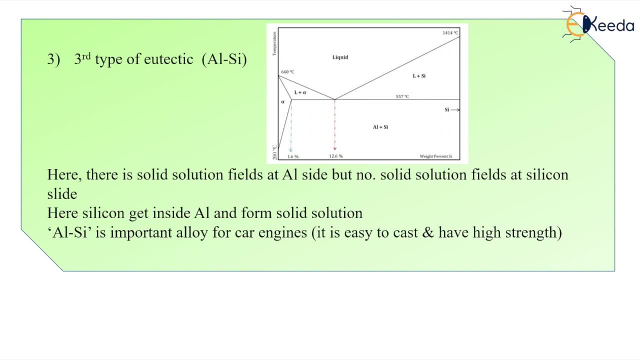 So, dear students, if we see this third type eutectic, we are getting in the aluminum and silicon alloy Here. you can see, here this is the phase diagram for aluminum-silicon. So this is a melting point of the aluminum and this is a melting point of the silicon. 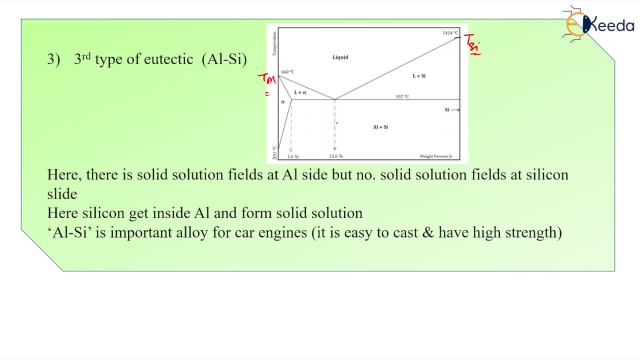 isn't it? So you can see, here only there is a solution field at the aluminum, isn't it? Aluminum side here, but no solid solution at the silicon side, No solid solution at silicon side. So here how actually silicon get inside of aluminum and for solid solution? 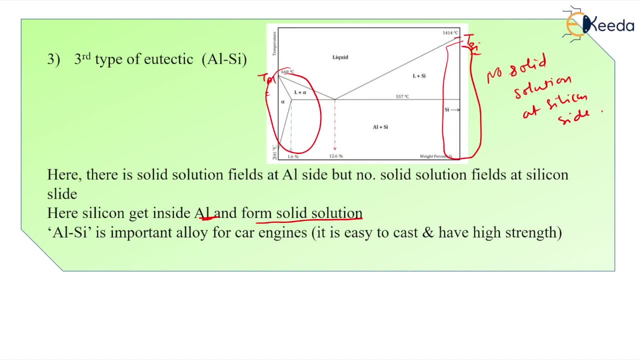 So, dear students, so this is the third type eutectic System, that is, out of these two elements, only one is having the solid solution. another is not having the solid solution. The famous example is aluminum-silicon alloy, which is very important. 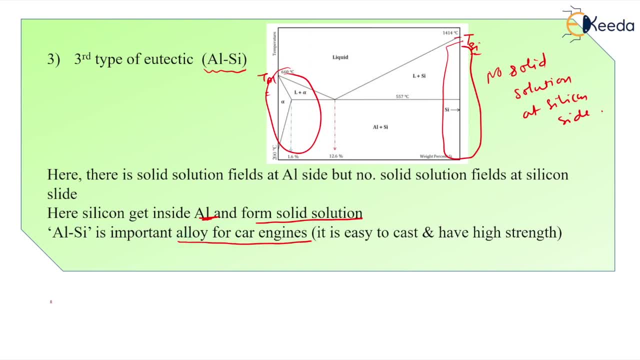 in the car engines, that is, it is very easy to cast and have a very good strength. This is most popularly used the alloy in the automotive sector or automotive industry For making the casting of this aluminum and silicon alloy for the car engines. okay, 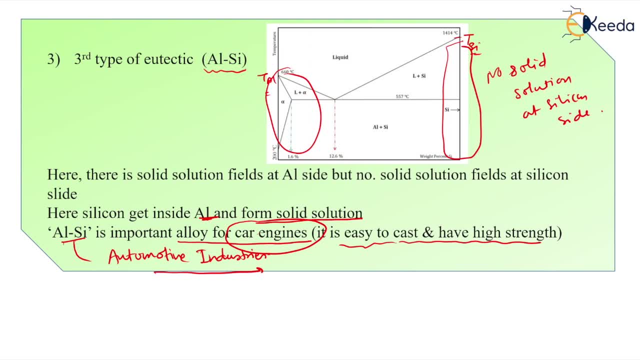 So this is the third type eutectic system. So very easy, dear students, if only one element having its solid solution, another is not having its solid solution, it is known to be the third type eutectic system. So, if you look at, actually, how the microstructure of this aluminum-silicon alloy, 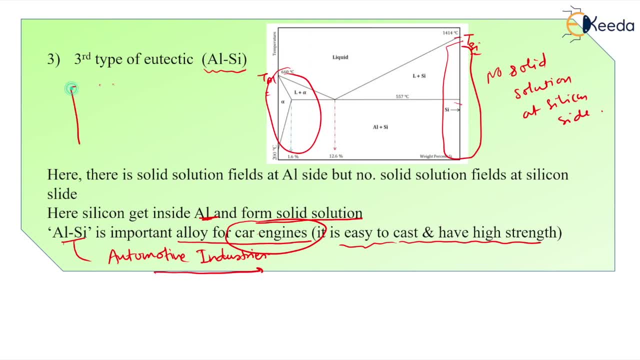 will see. So, if I show you here, there will be the white, this matrix, this background is of aluminum, okay, and there will be the needle-like structure of like this. There will be the needle-like structure of this silicon.